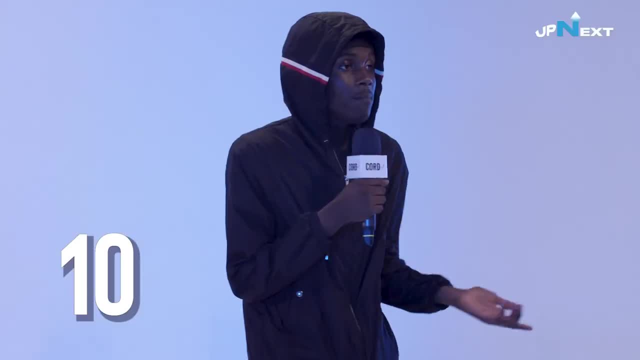 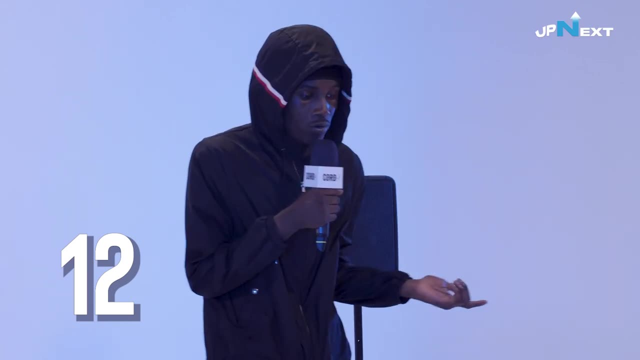 i think about nine. i'm missing my slam. he's looking at ten- attempted a murder again. he's up in that prison with most of my friends. when we was 11 we said 12, we're cutting from them. it's numbers. when i blow one tree, she asking you the one for me, dtb. since i hit 15, 16, stepping. 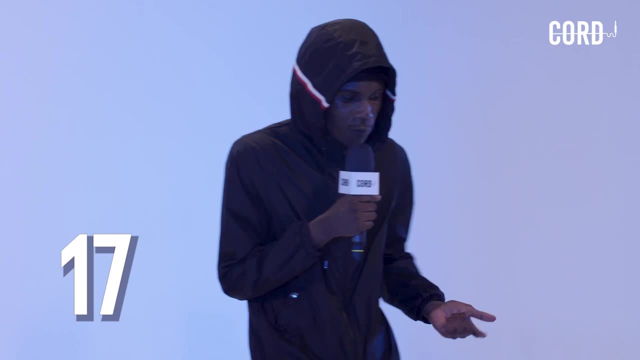 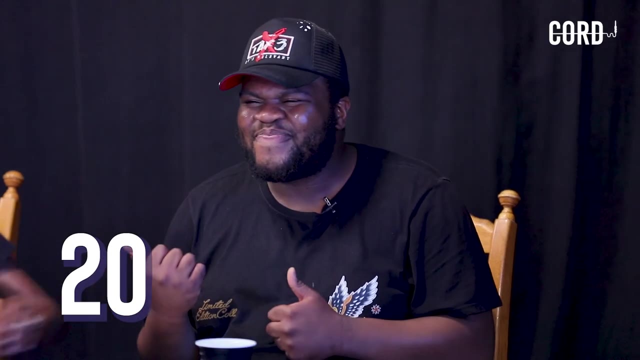 consistently resided in the 017. it fell on just before 18.. half my age would have been one nine long time since i lost the fight. now i'm like 40 going on 20. advanced, i can't deny fifa and i'm 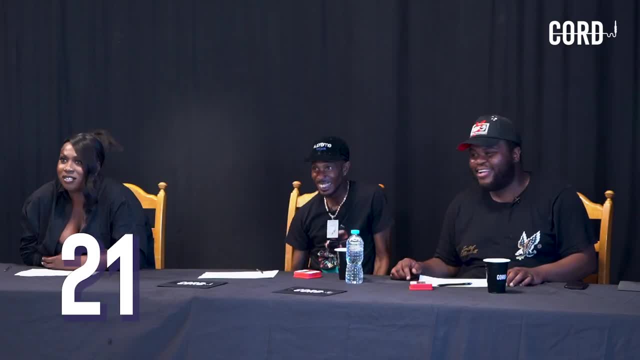 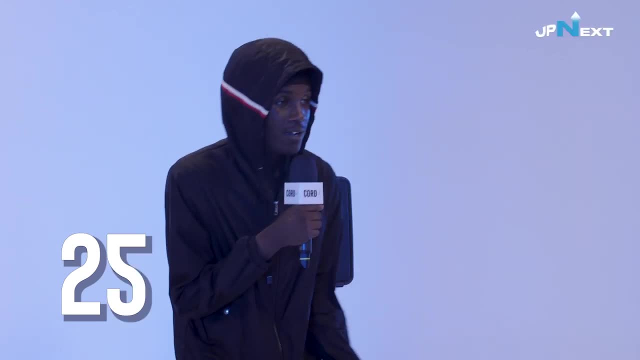 up 2-1 and it ain't even hit half time. half-pipe 22, then two freeman. i'm not surprised. 24 seconds for me to dump thing quick. now he's looking at 25.. it's alive by 26. can't be in the mix. 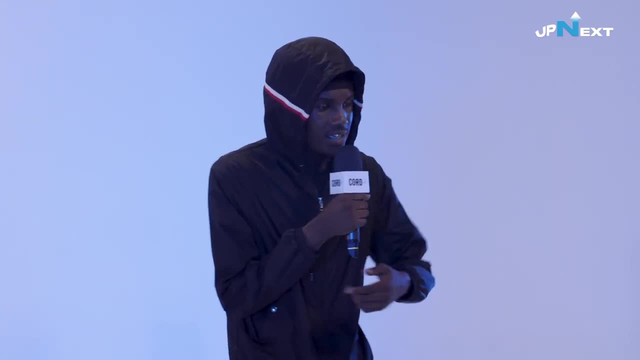 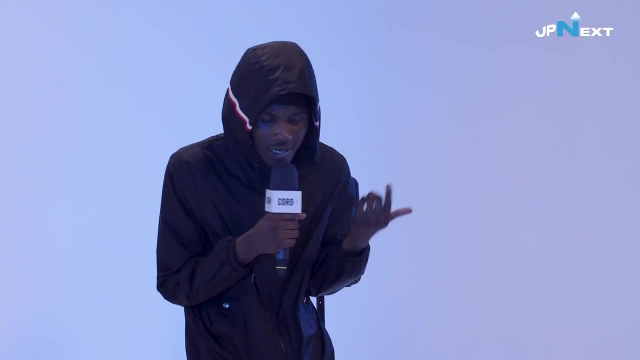 you. if you put me in a room with a mic, i'm burning. i don't care about girls, they already hurt me enough. man, switch lanes. i'm sturdy enough sometimes when i lock myself in the booth cause i don't really feel like they hear me enough. but i, 26, can't be in the mix used to. 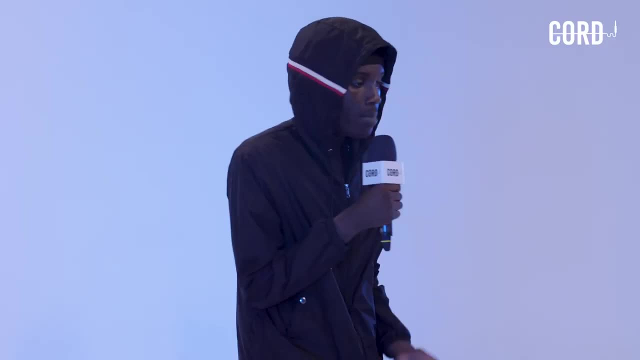 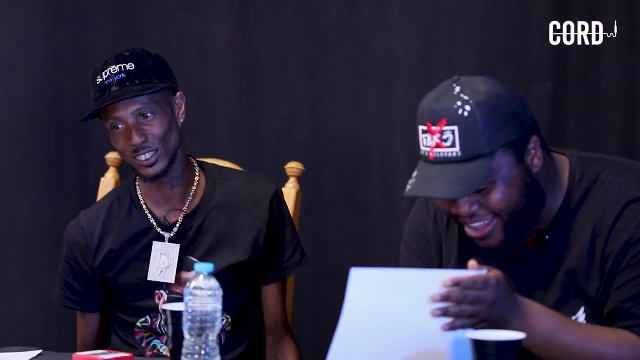 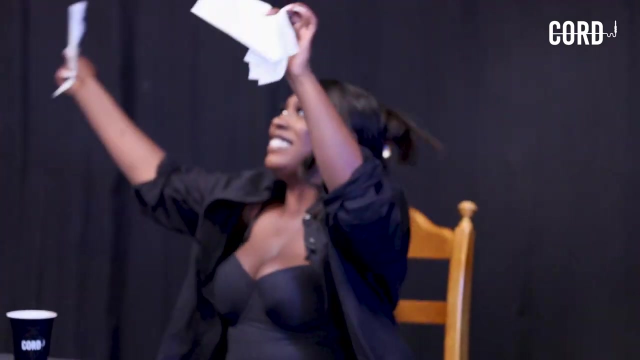 ball galactic. if you put me in a room with a mic, i'm burning it up. i don't care about girls, they already hurt me enough. man, switch lanes. i'm sturdy enough sometimes when a lot myself in the beef car don't really I don't know what to do. 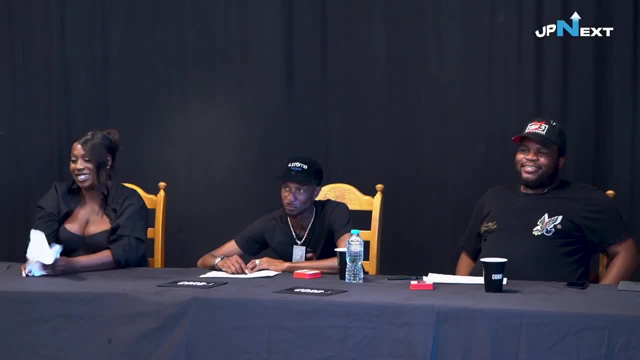 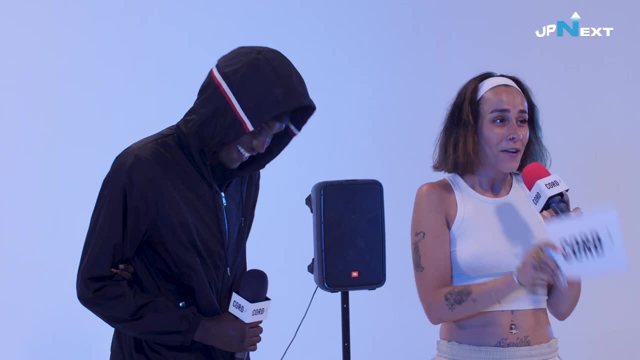 I don't know what to do. I feel like I need to remind the judges. I feel like I need to remind the judges that there is seven people you've got to watch and there's only three you can put through. and this is number three and all one, two and three. 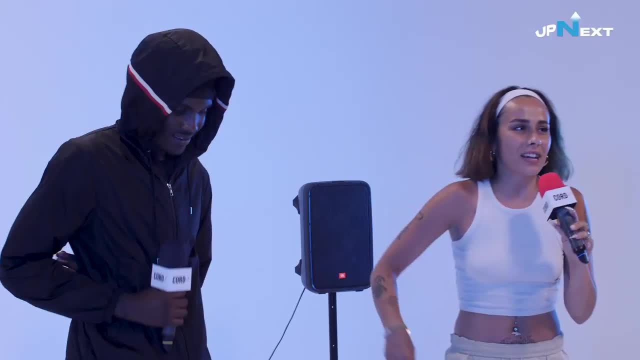 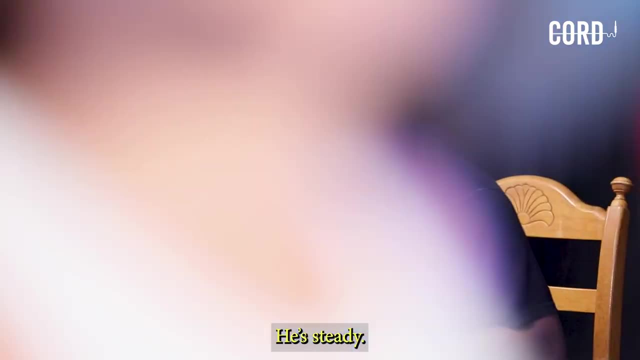 have apparently rocked your boats. so let's hear it for Twice one more time. He's good, He's confident. If he's Twice, he's the one I can live with.